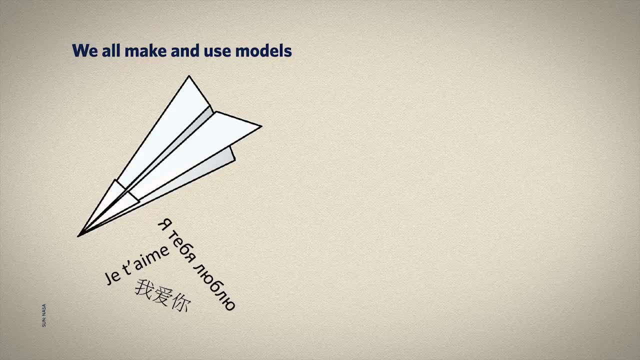 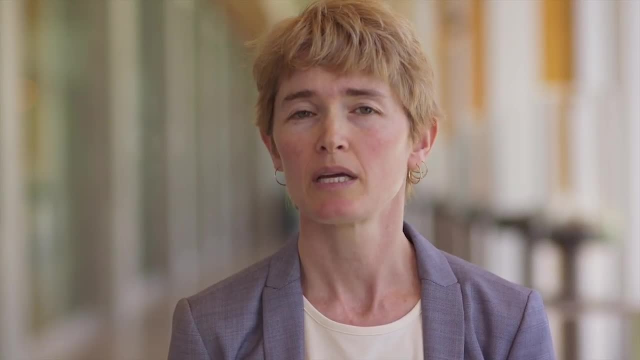 Though in our language we do aim to get as close as possible to communicating what it is that we're thinking. We use physical models in architecture to show what something might look like if we were to build it. We use models in engineering to test designs before putting the time, effort and energy into building the real thing. 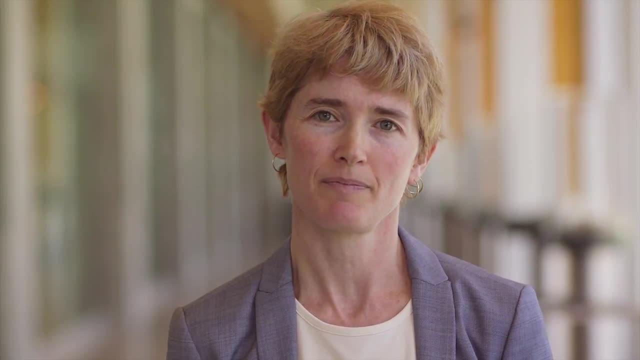 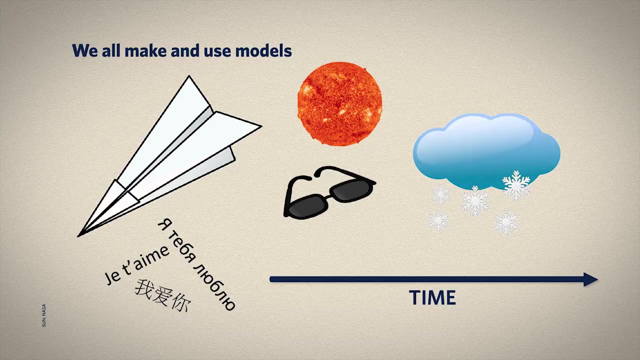 We even model our own futures ourselves, And our models help us plan ahead because we have expectations of the future. We expect, for example, that next winter will be colder than the following summer. We might not know exactly how cold or how warm the seasons next year will be. 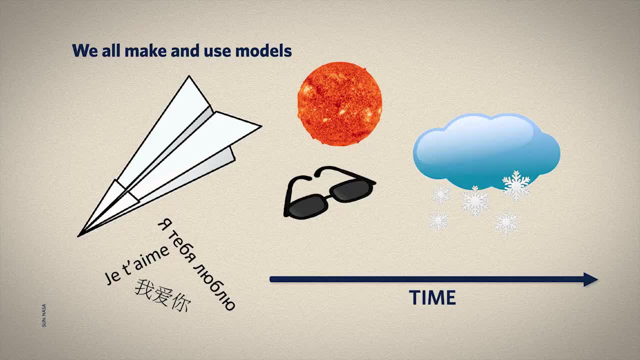 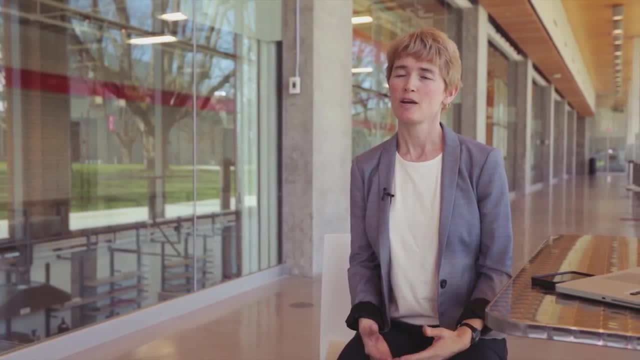 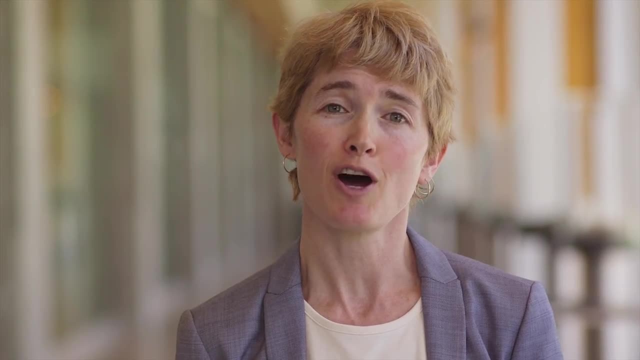 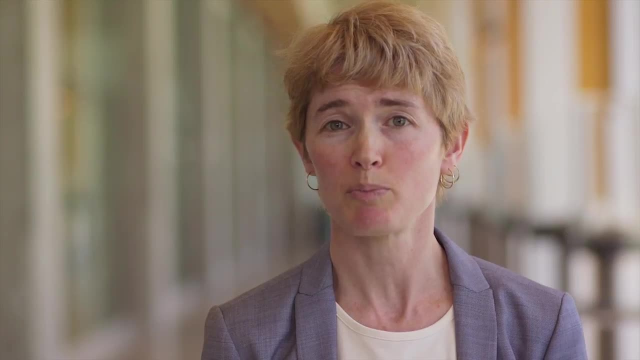 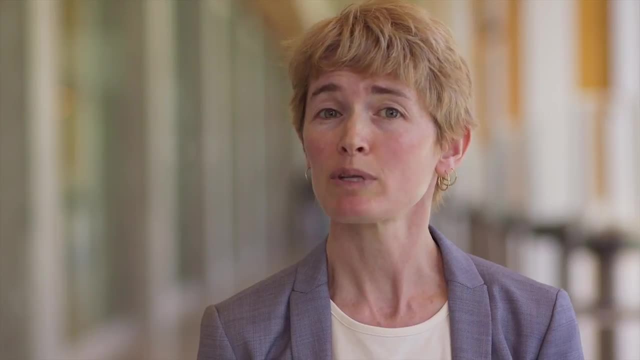 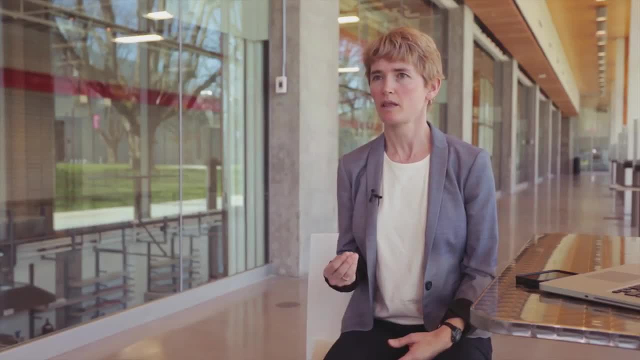 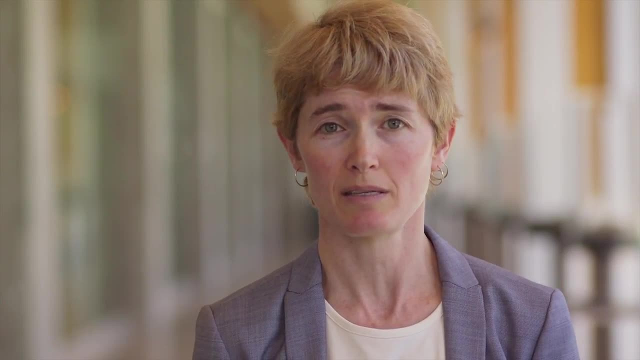 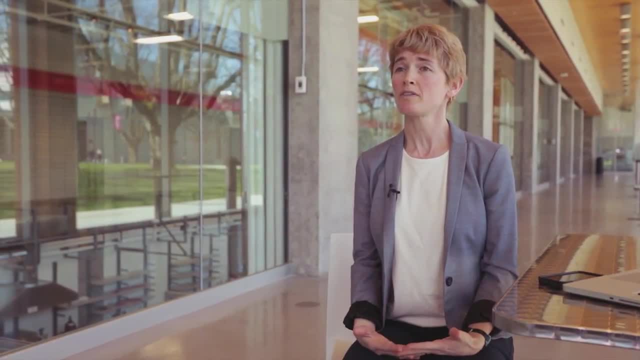 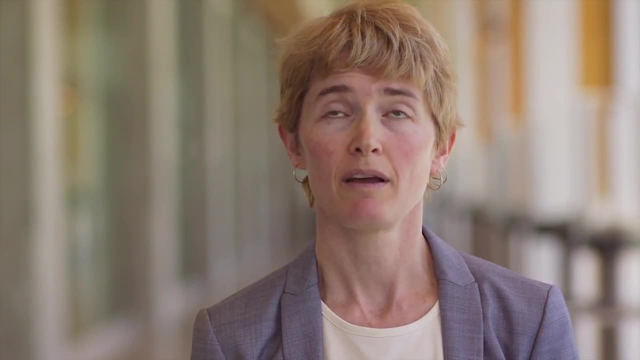 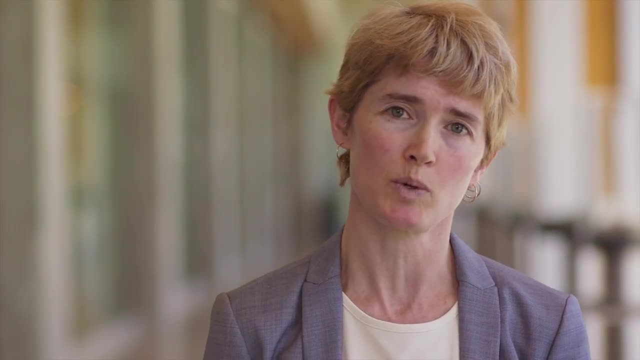 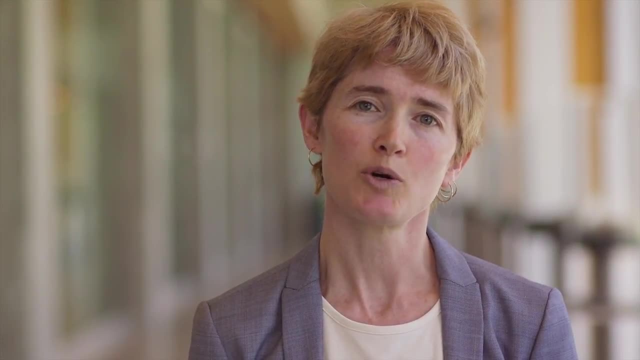 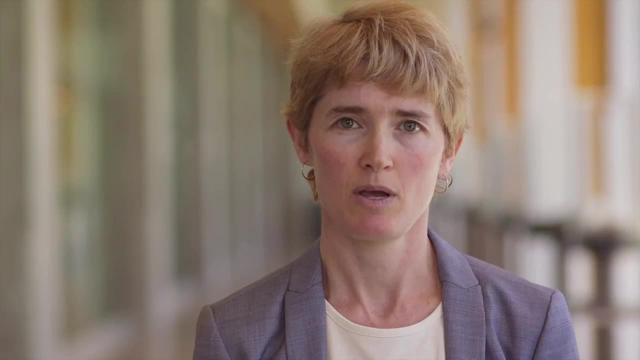 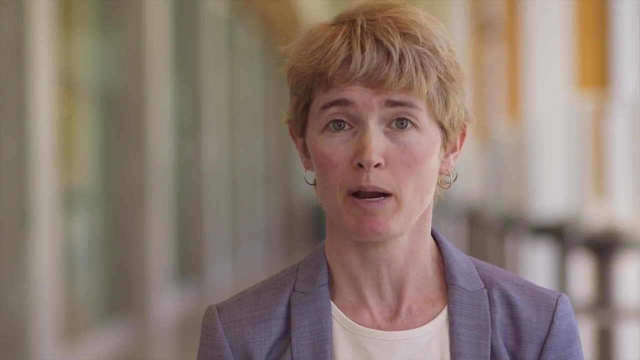 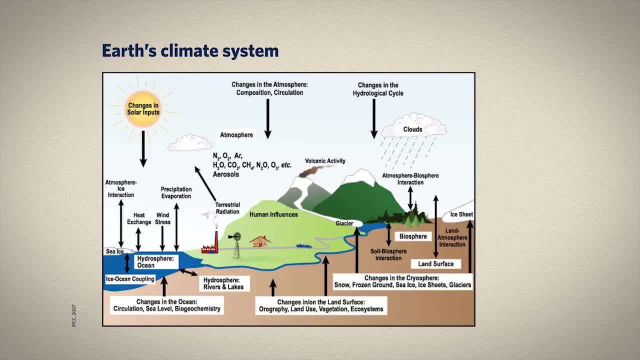 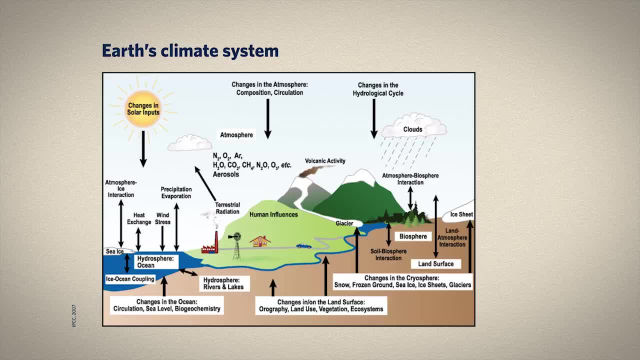 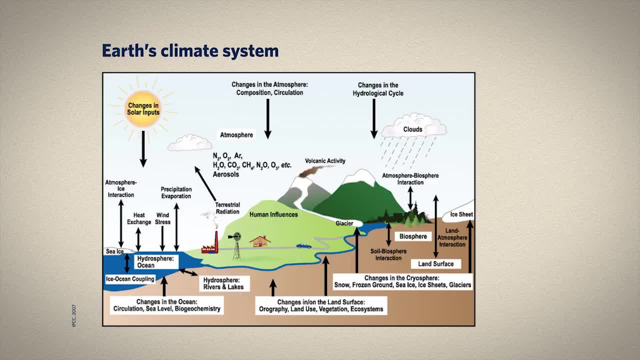 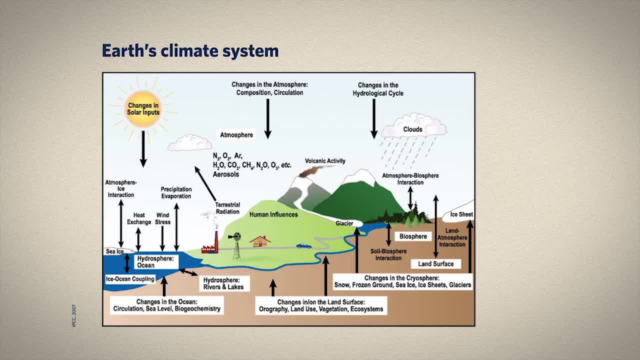 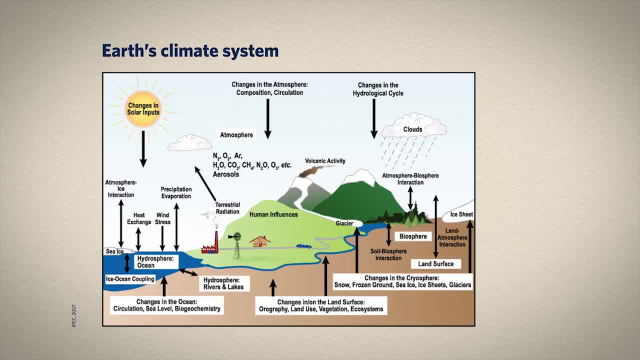 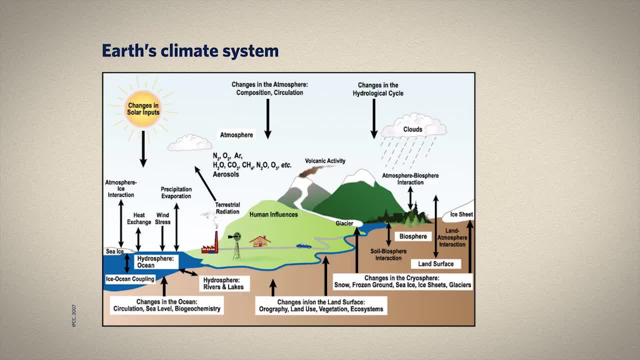 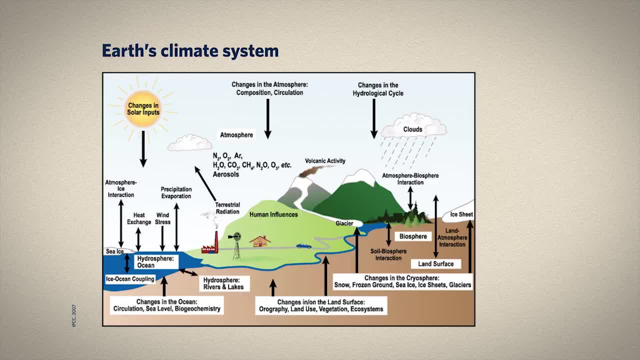 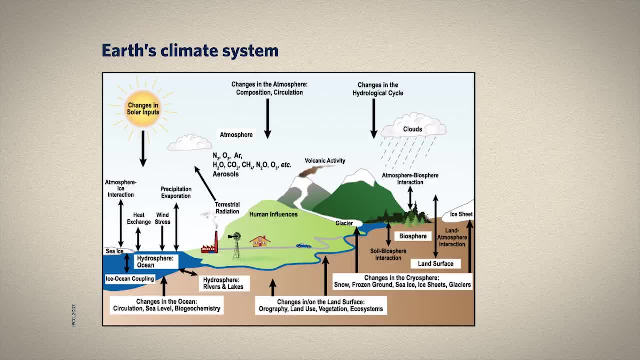 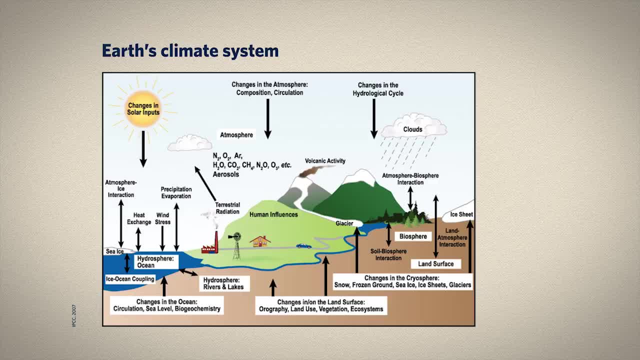 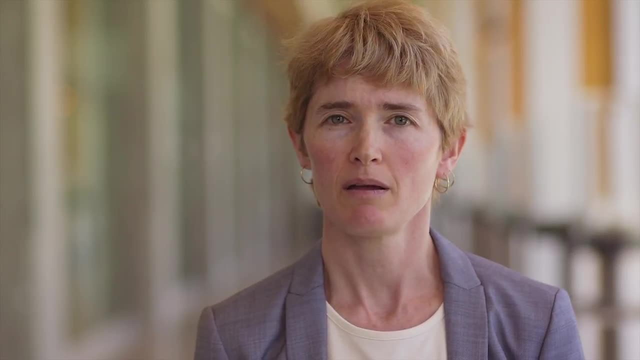 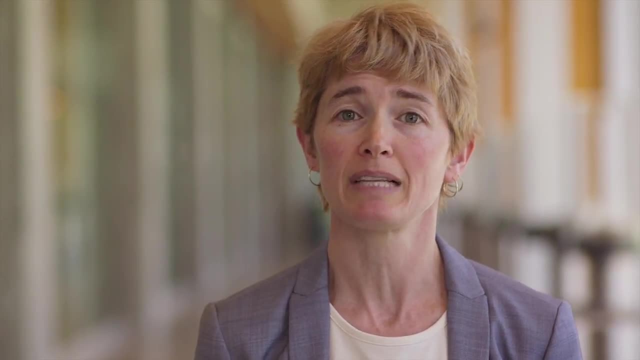 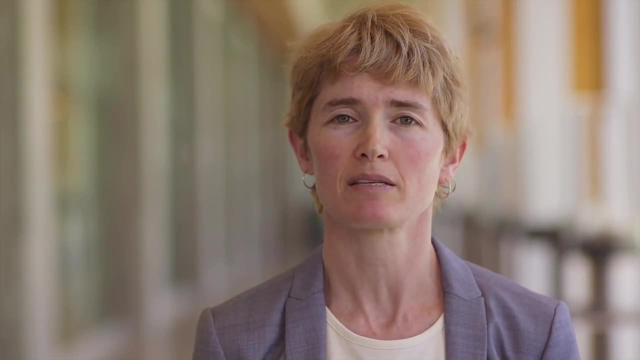 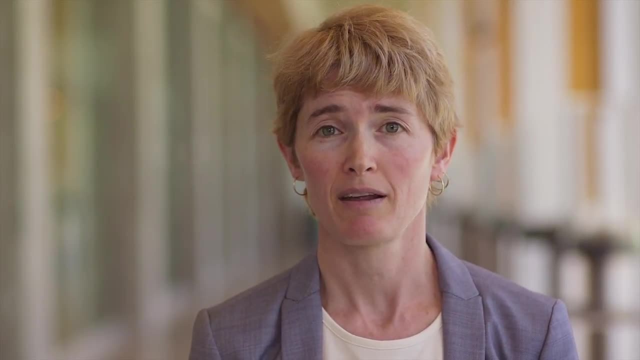 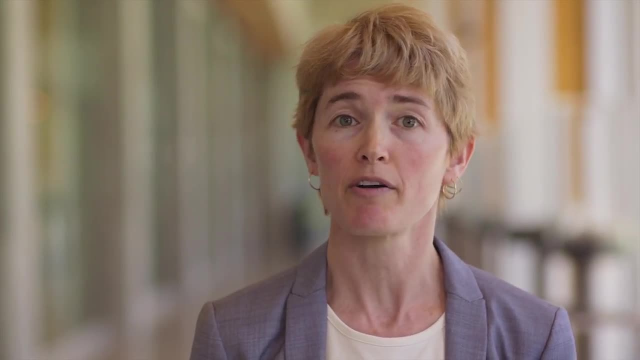 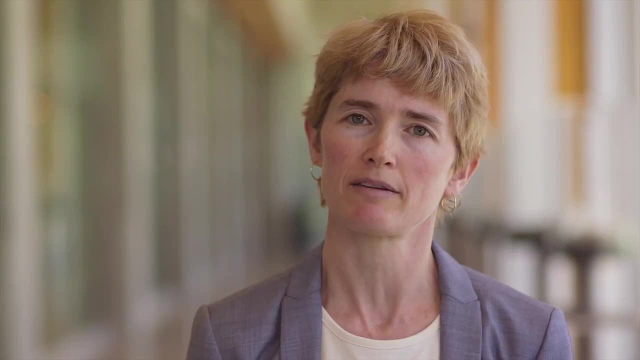 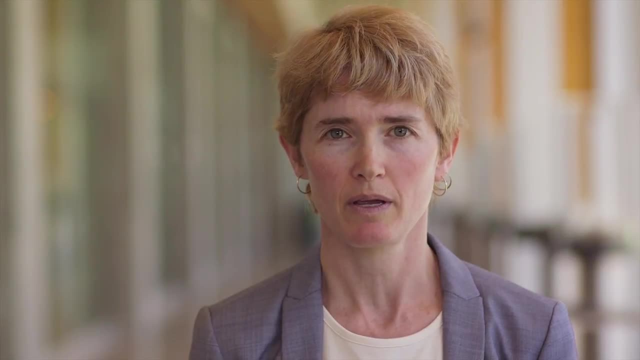 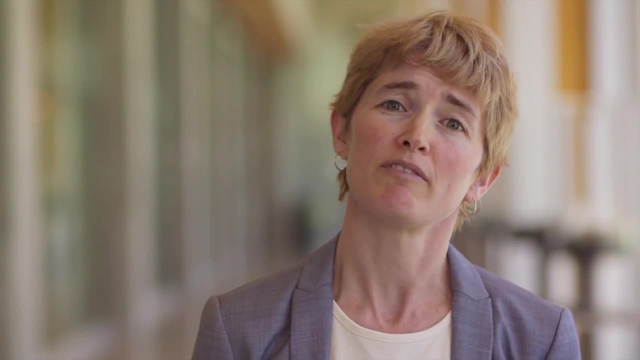 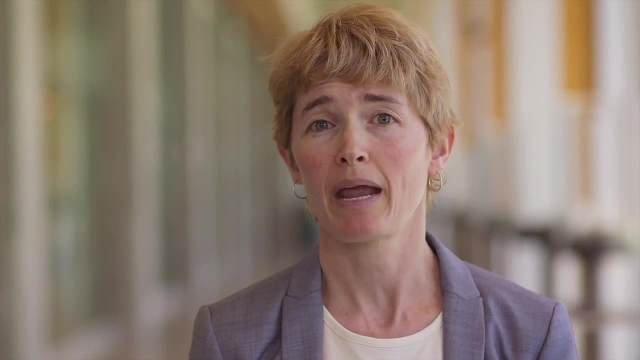 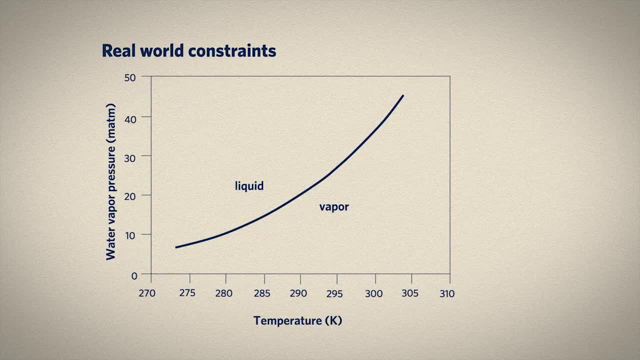 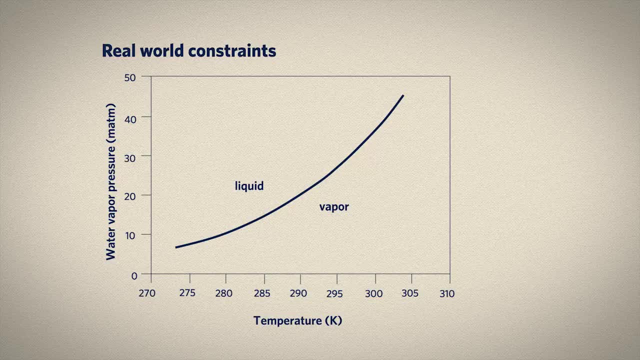 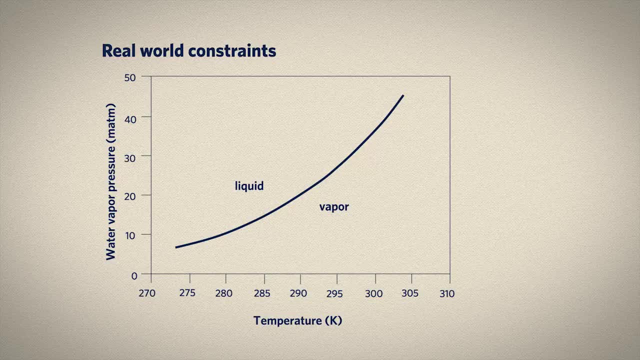 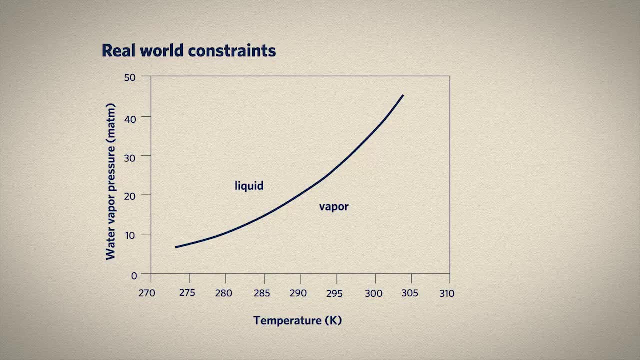 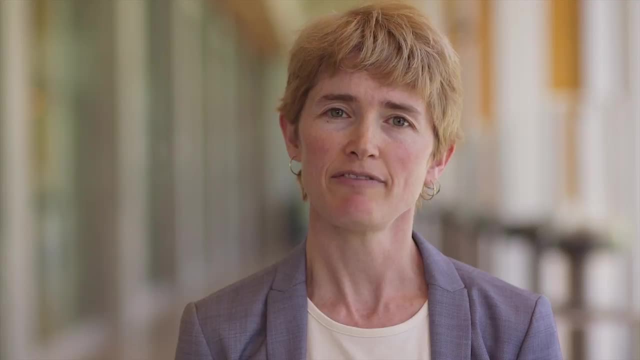 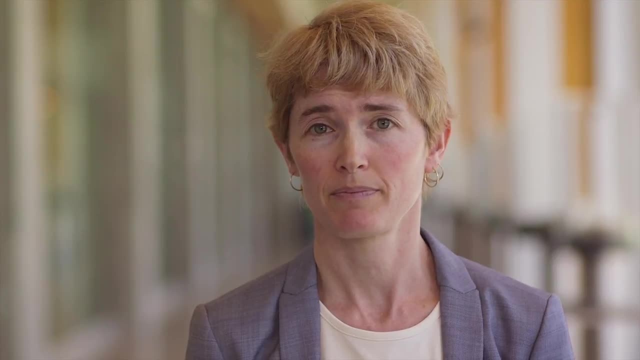 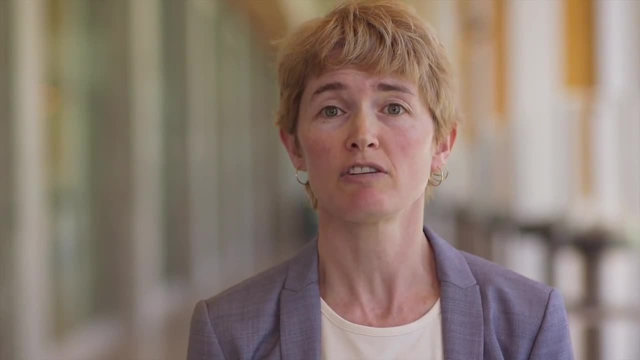 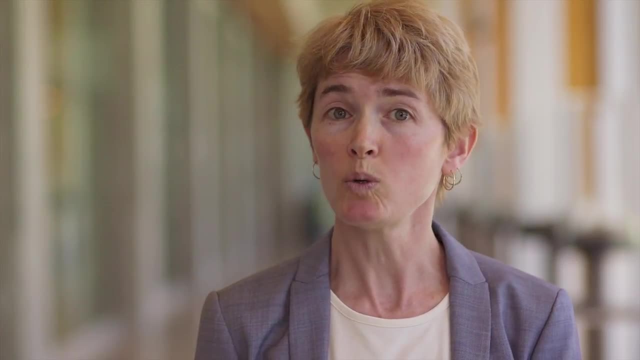 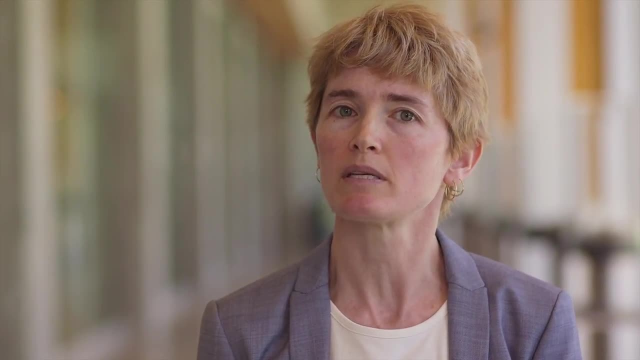 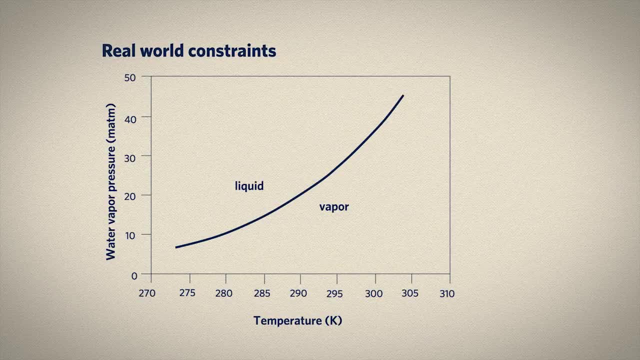 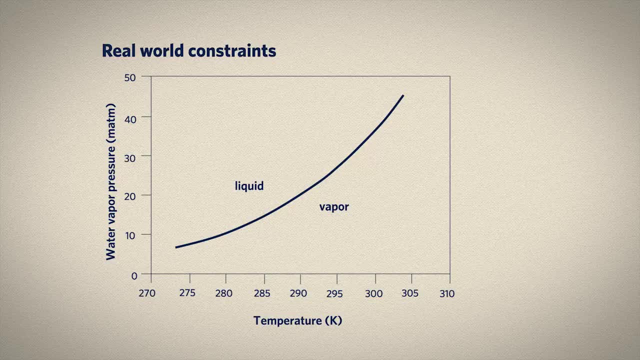 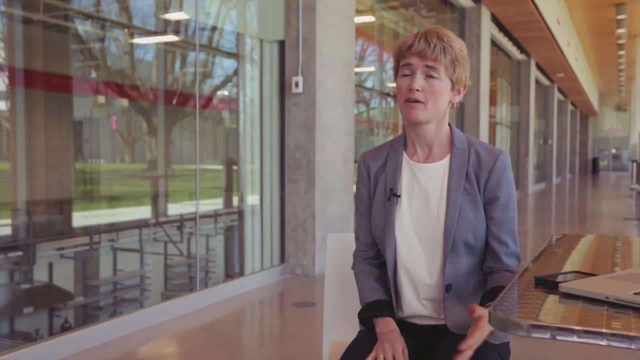 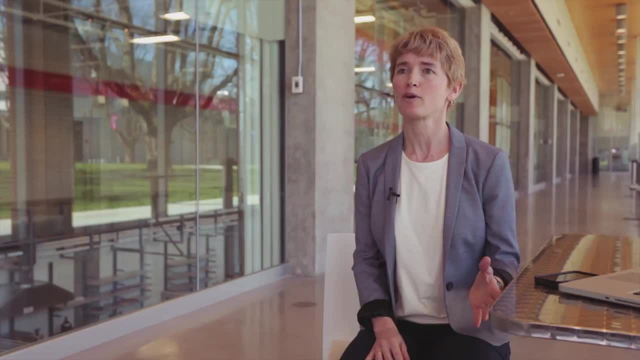 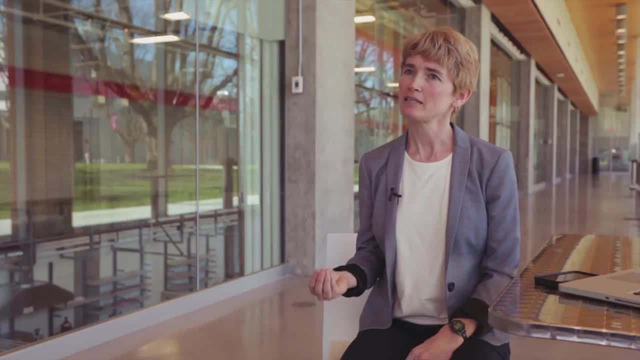 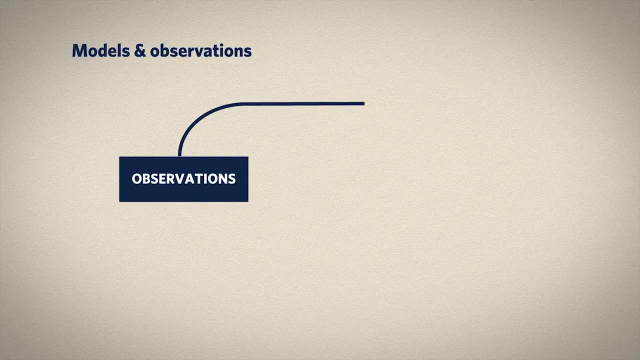 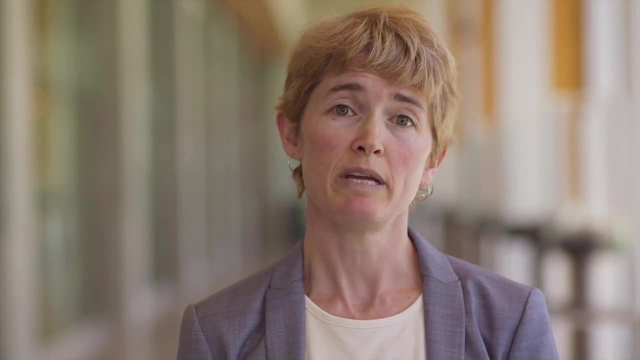 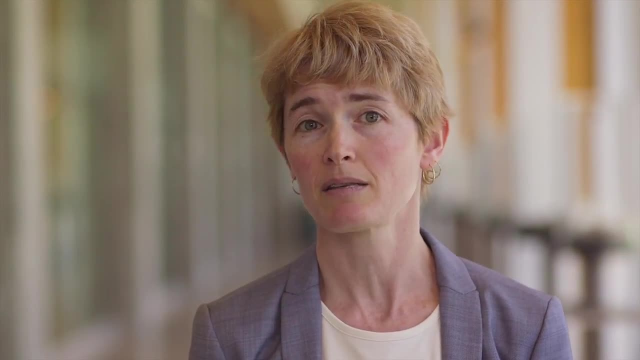 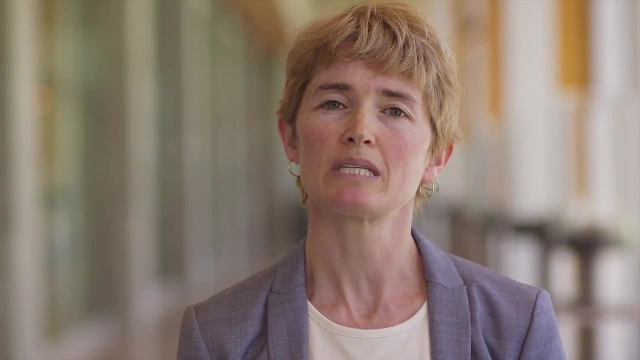 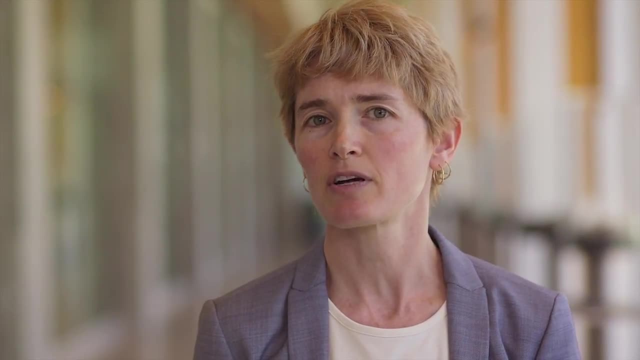 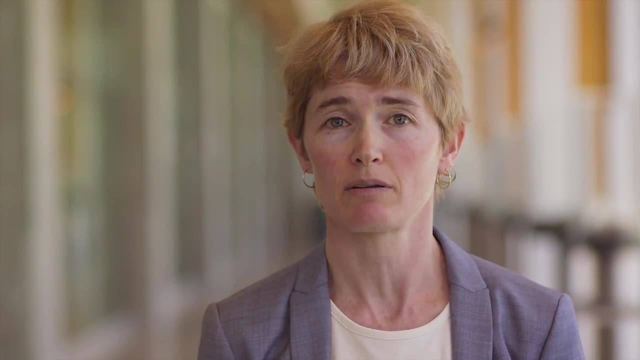 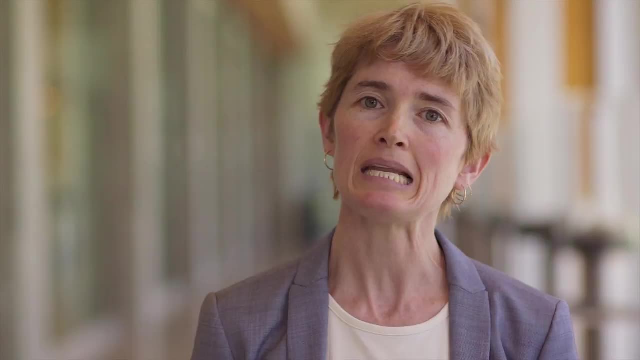 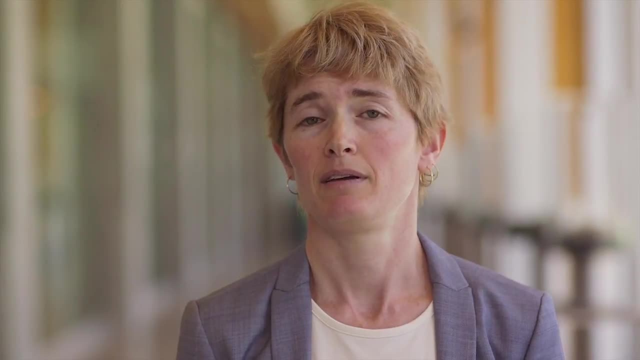 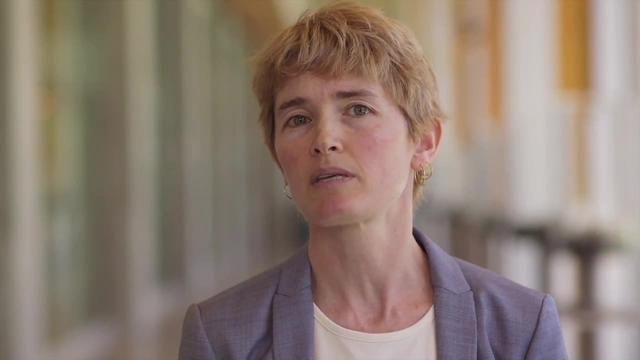 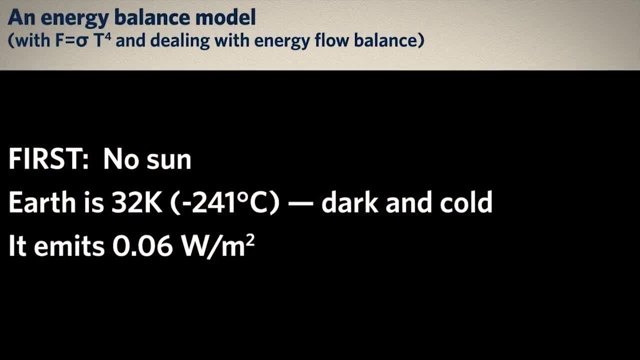 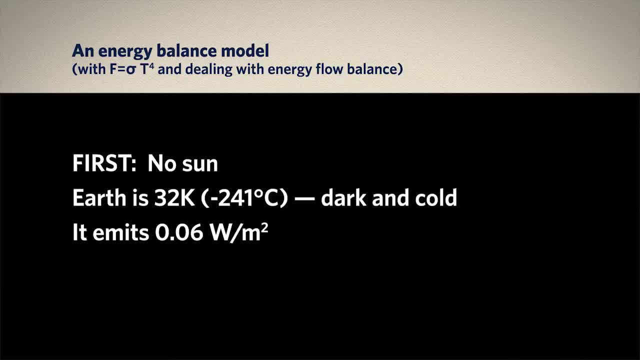 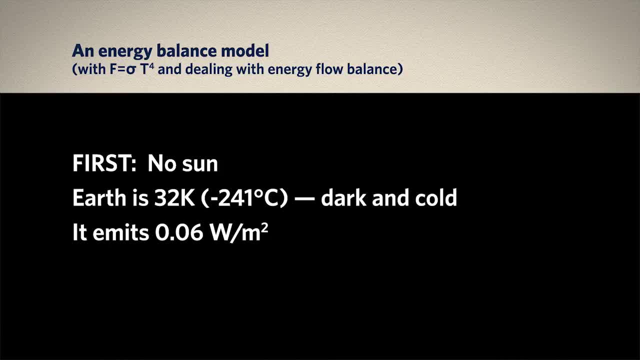 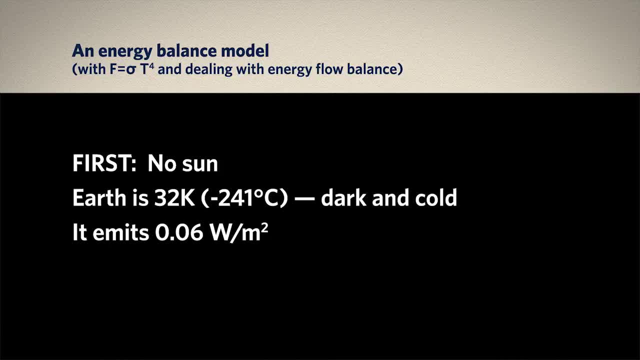 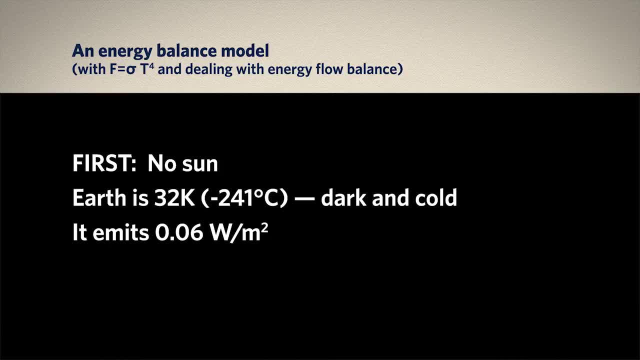 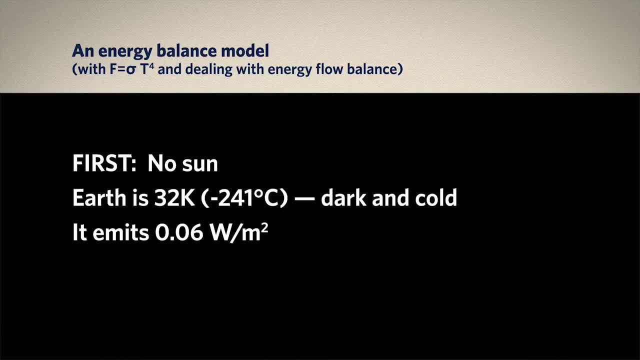 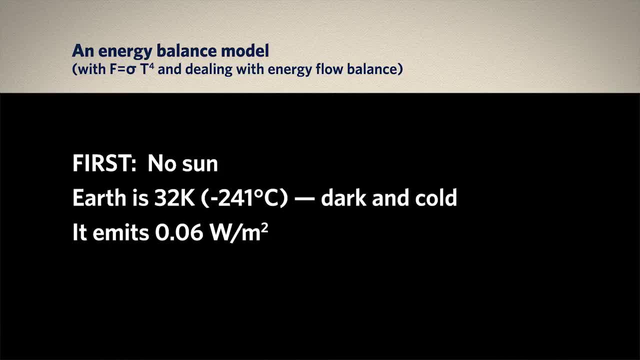 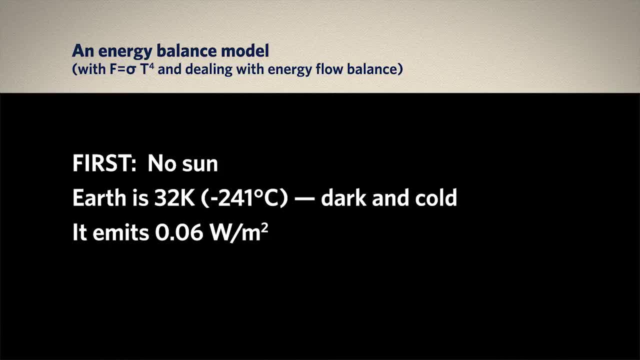 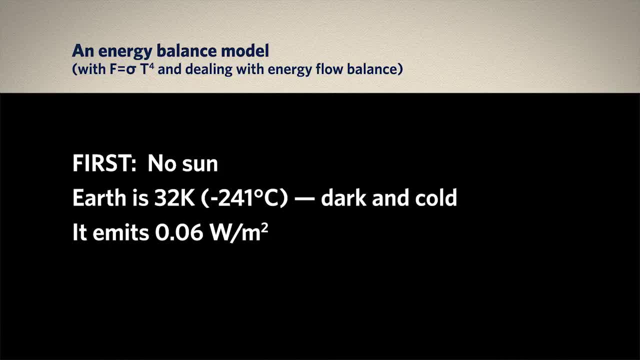 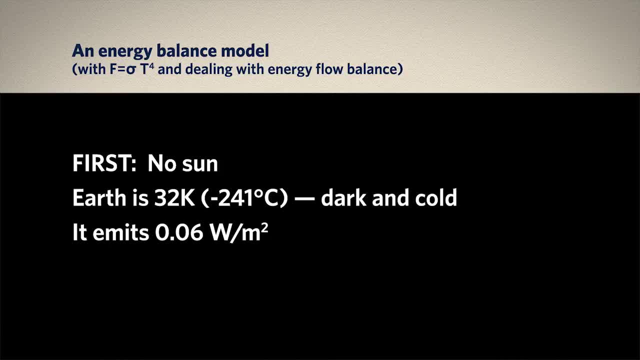 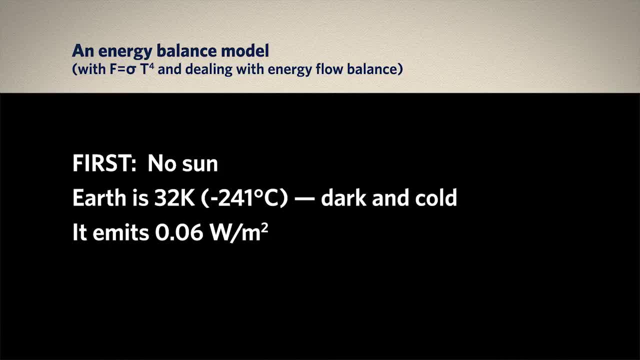 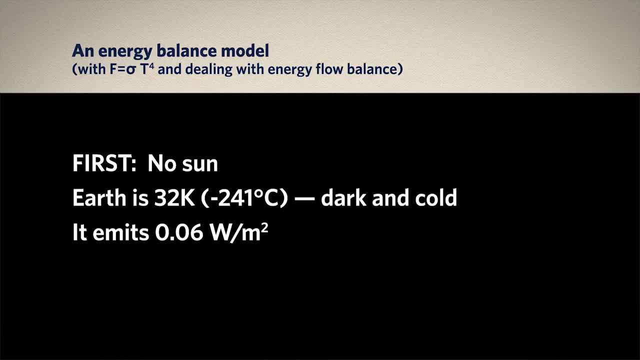 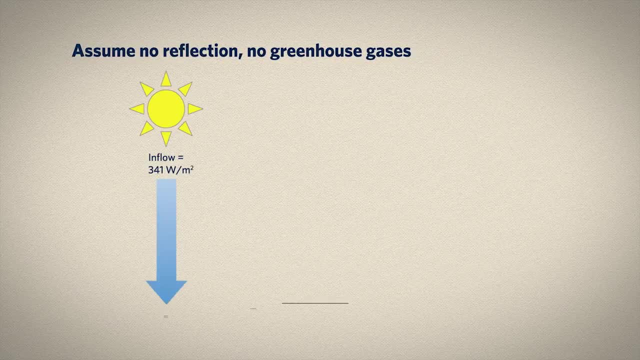 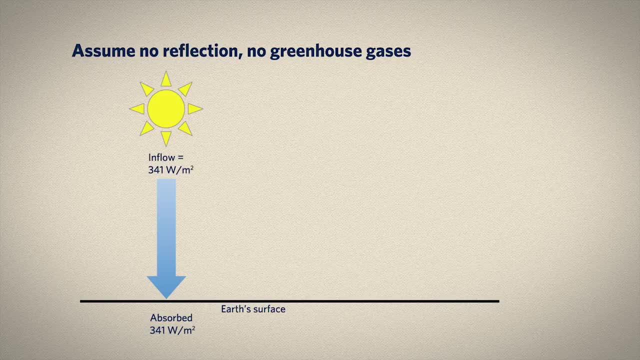 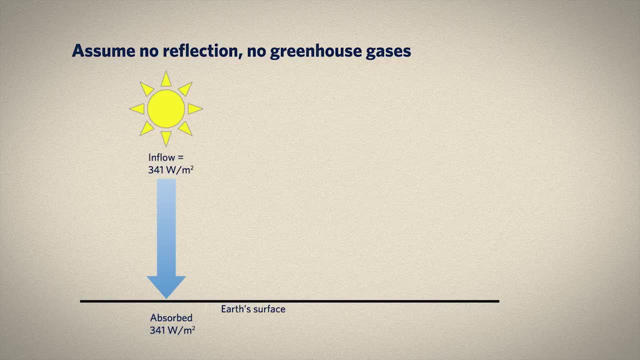 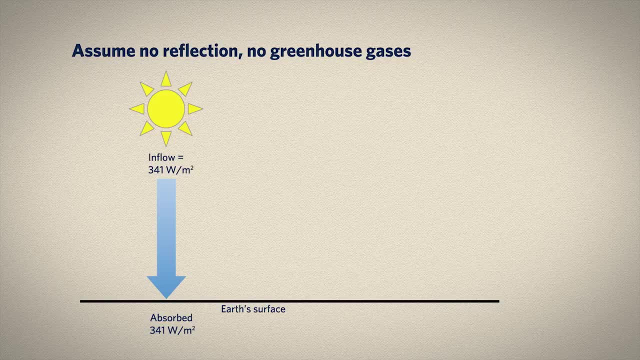 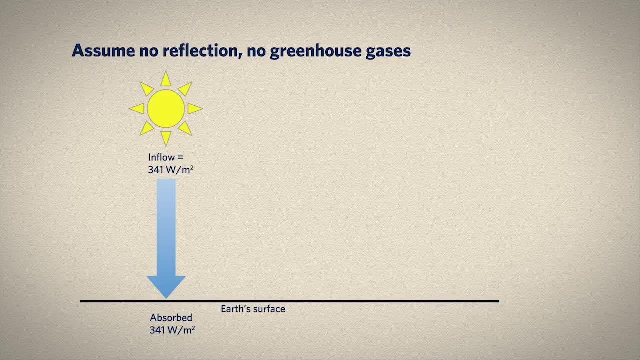 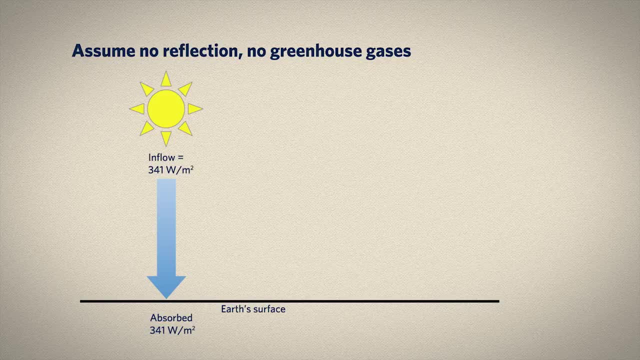 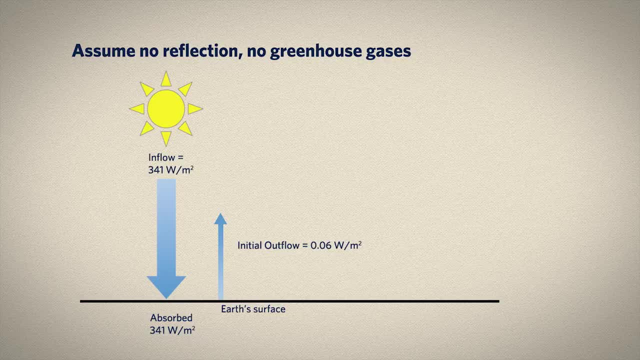 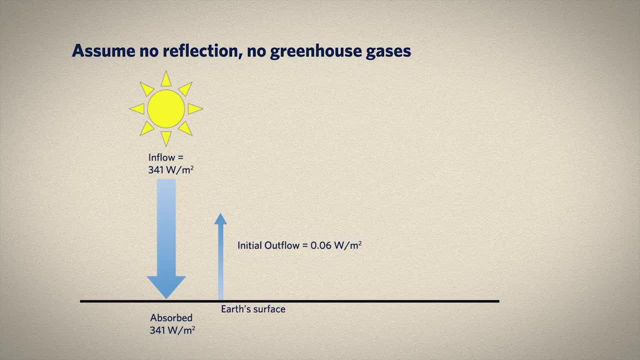 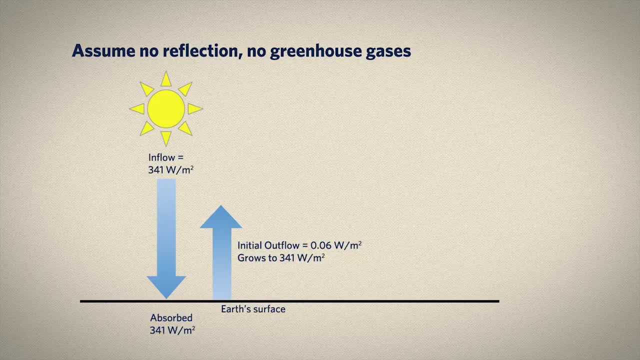 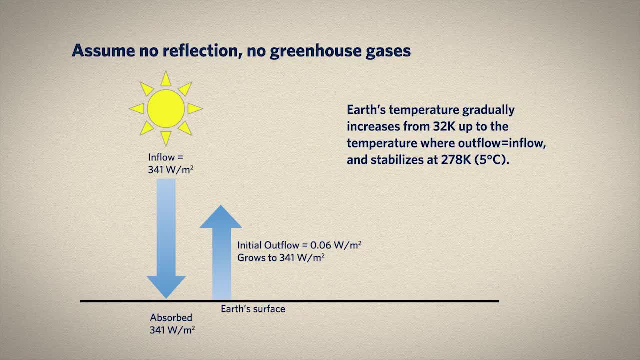 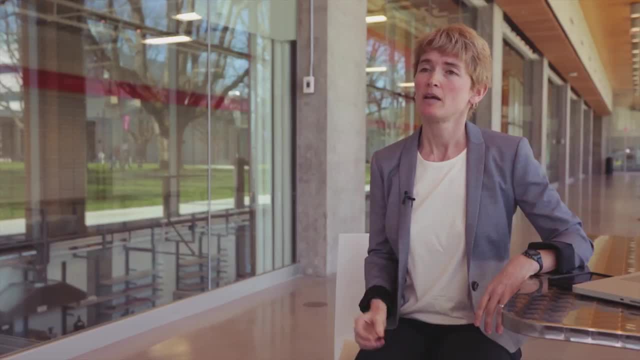 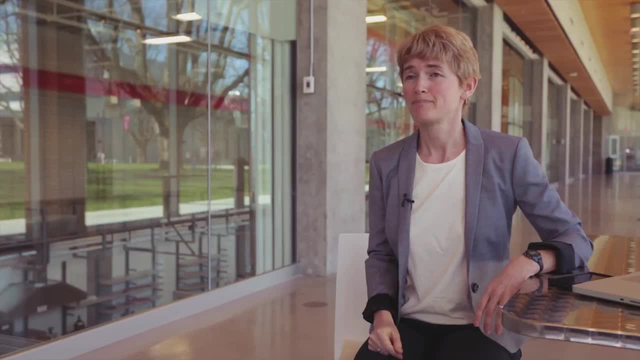 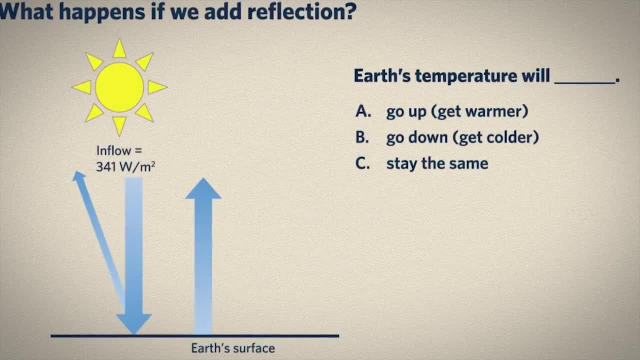 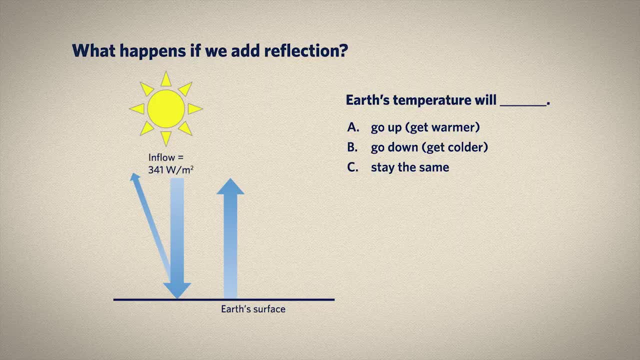 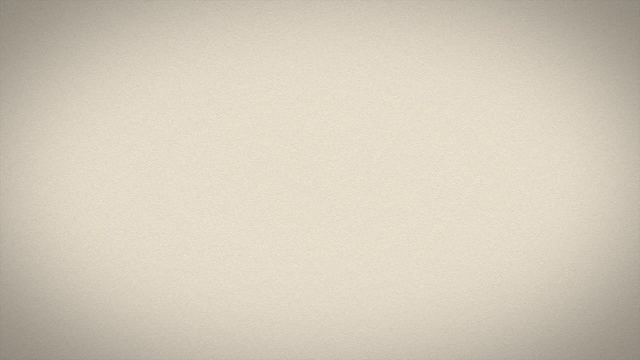 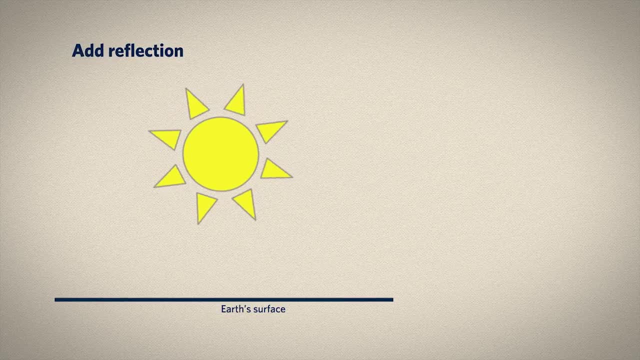 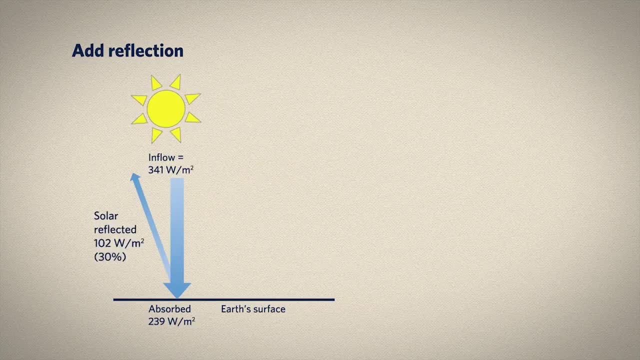 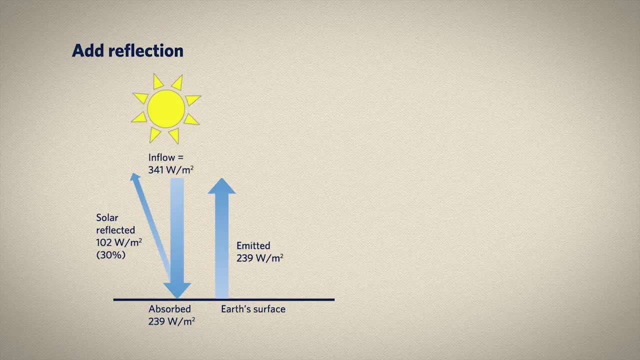 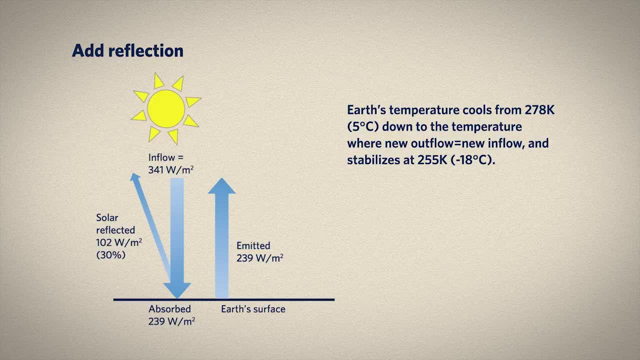 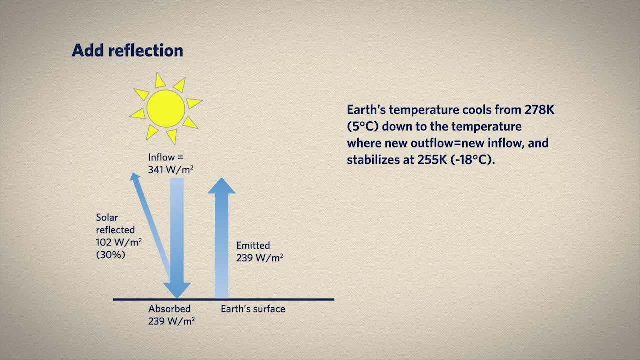 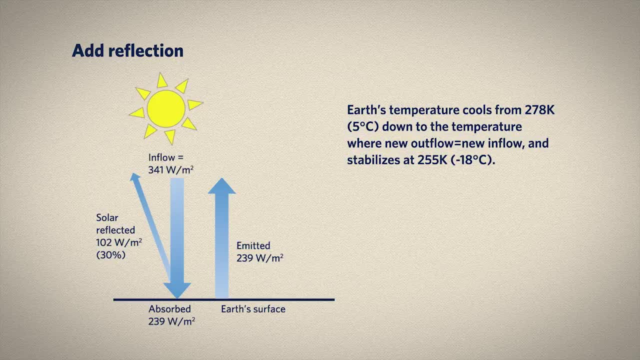 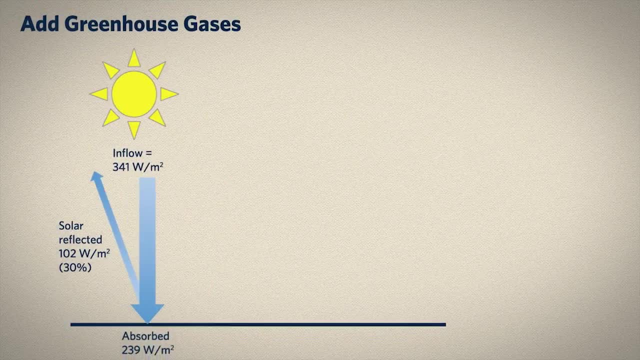 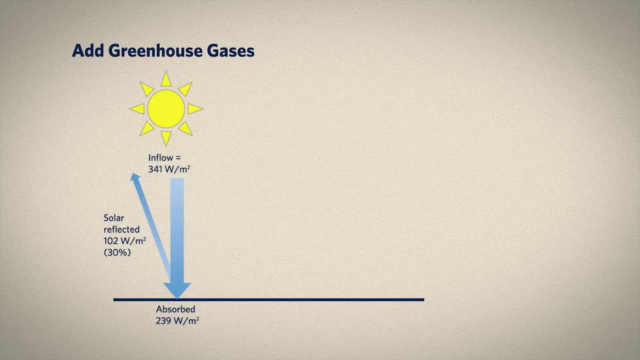 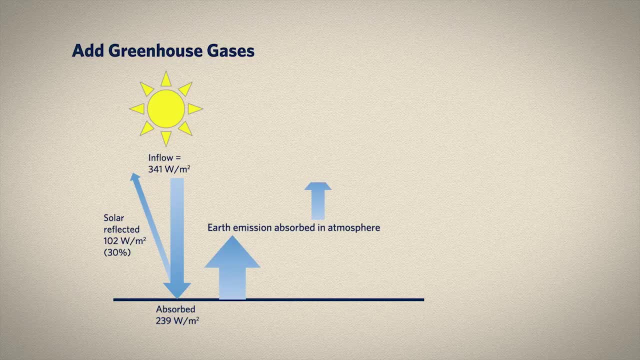 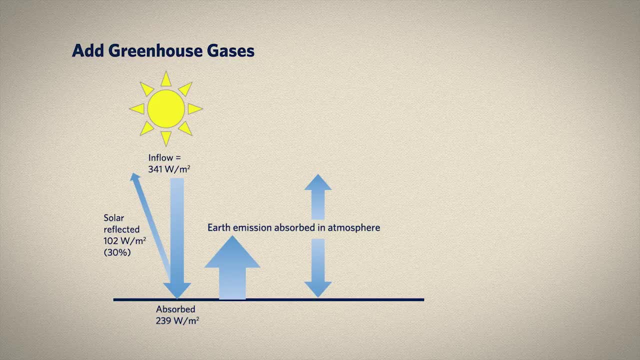 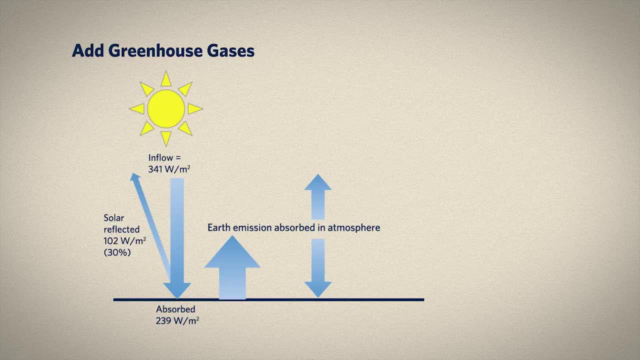 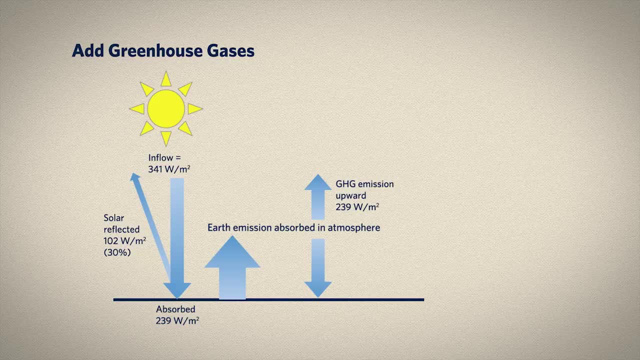 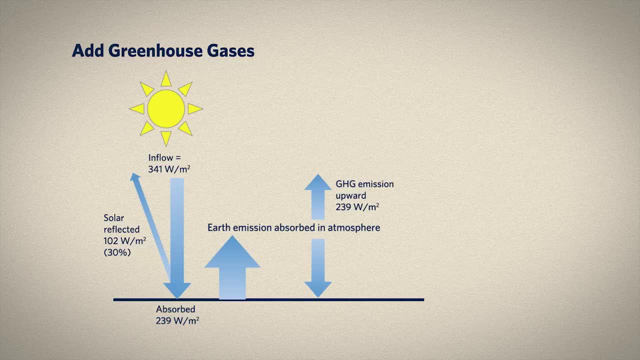 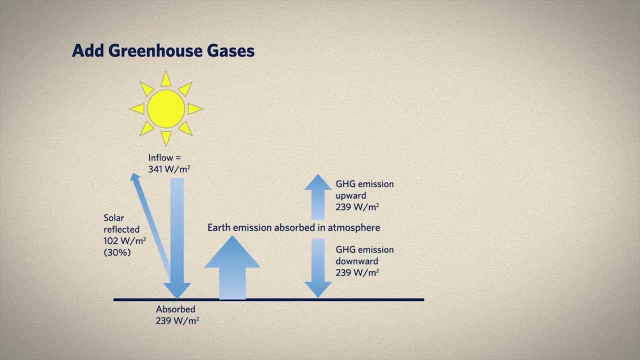 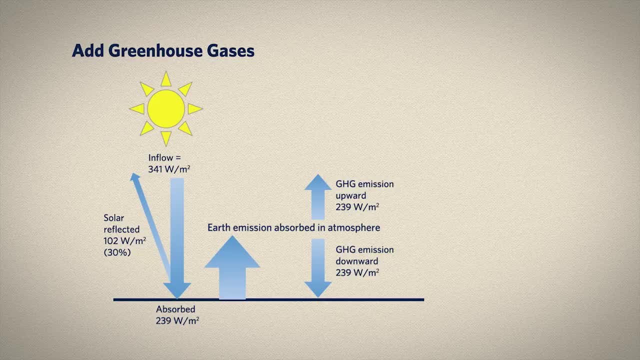 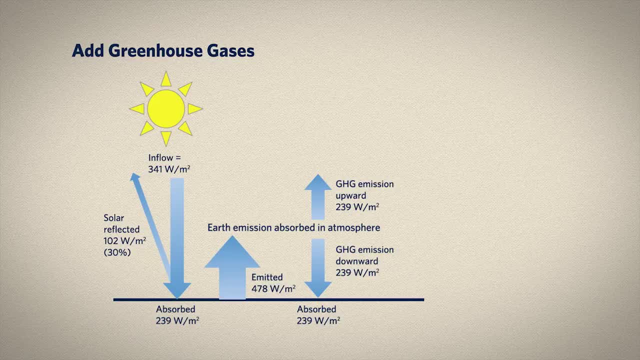 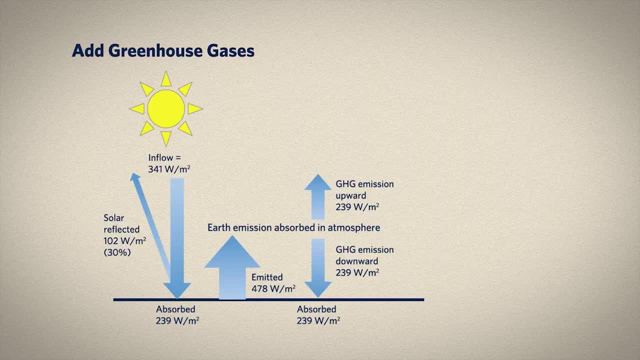 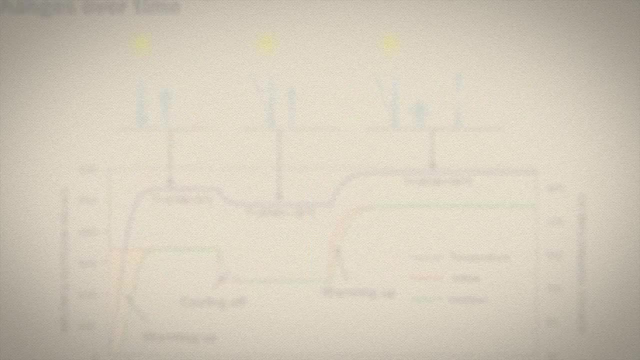 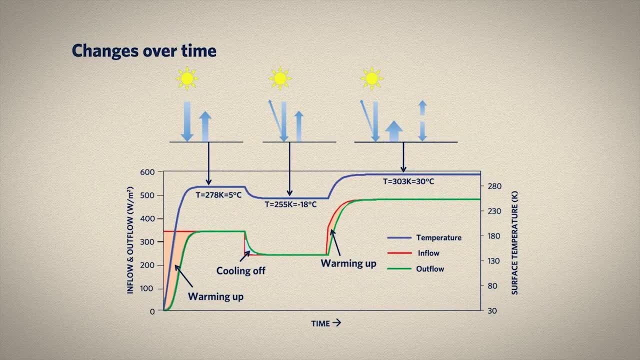 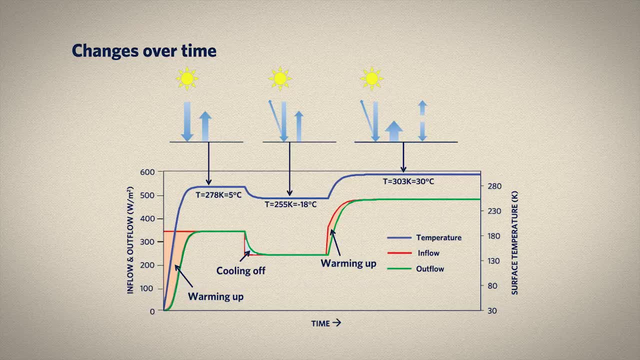 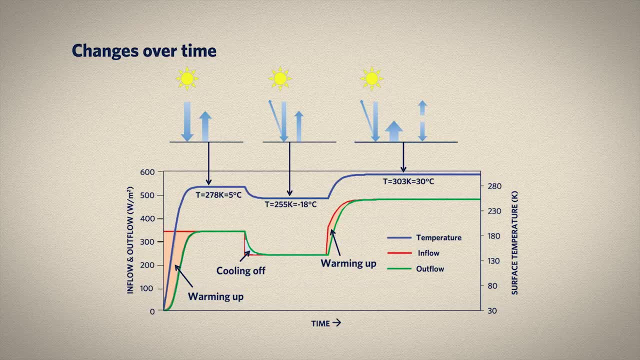 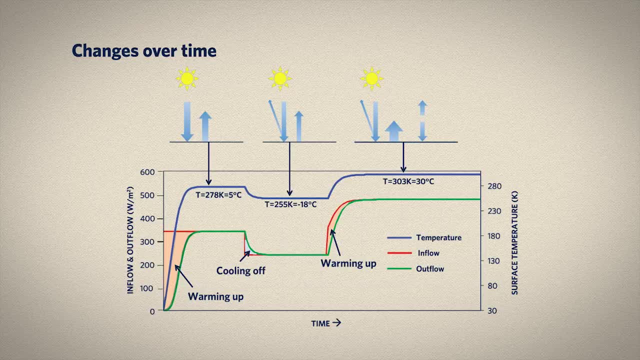 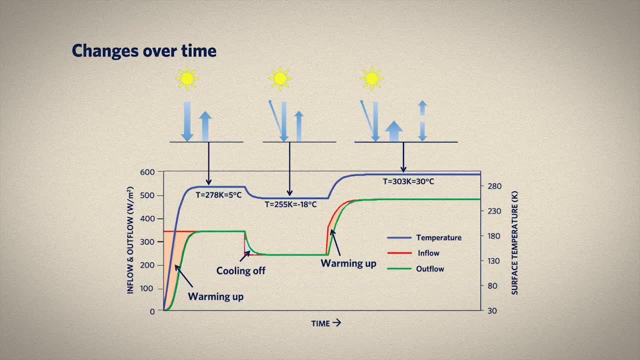 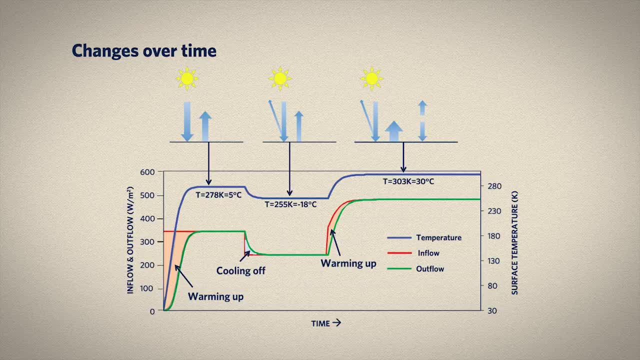 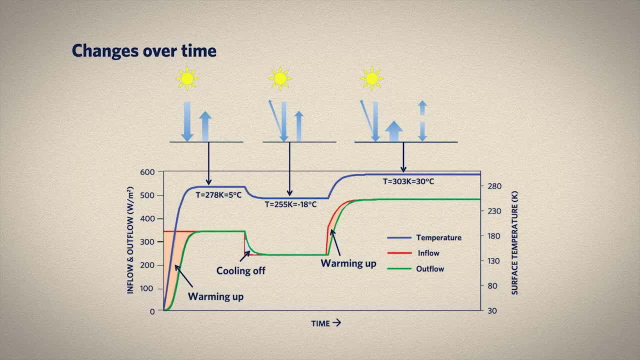 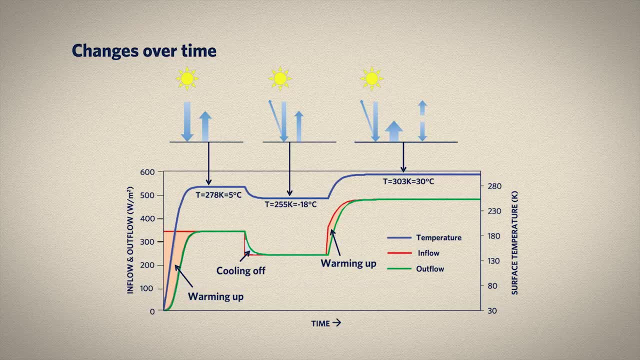 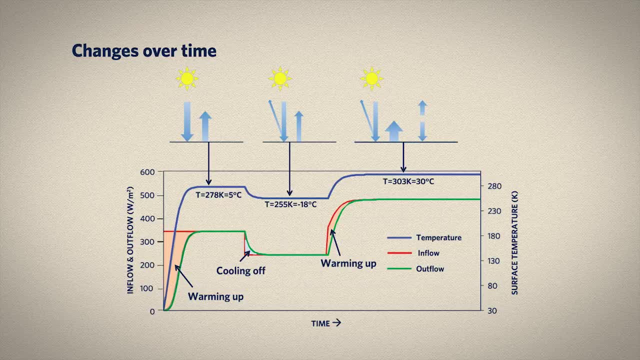 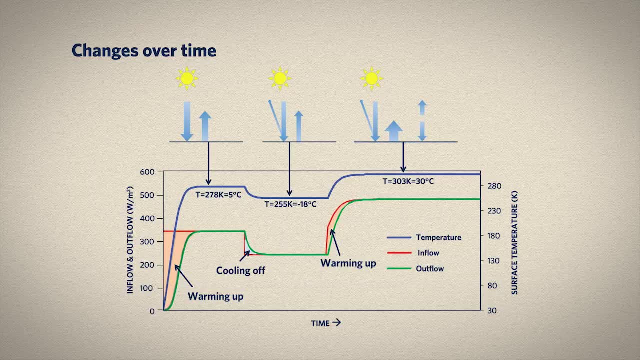 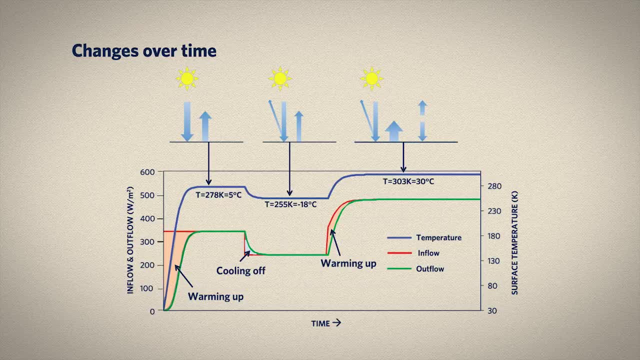 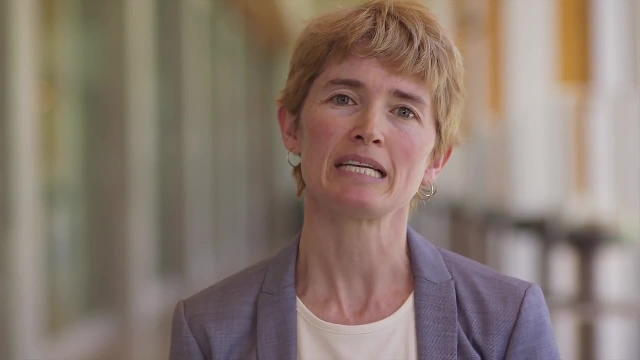 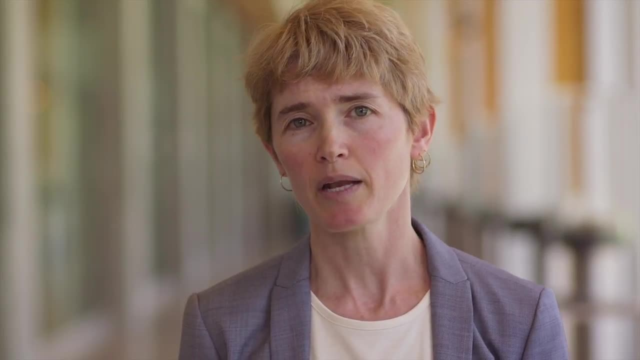 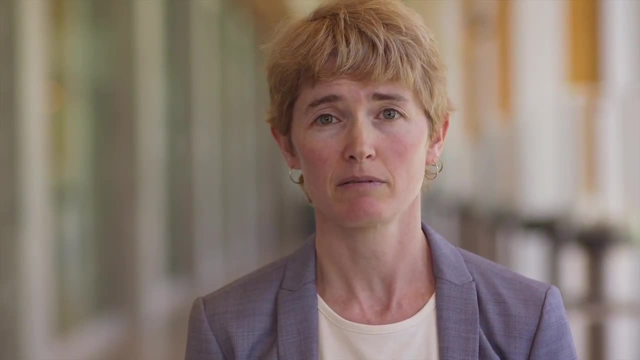 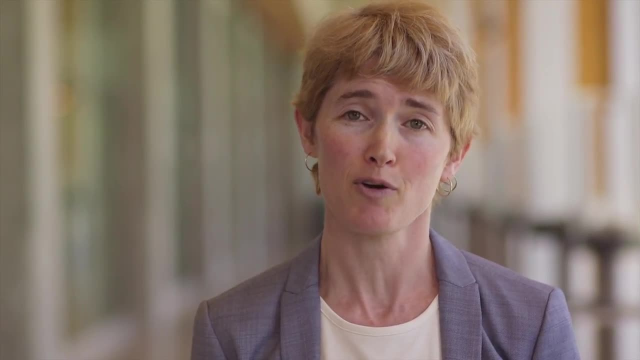 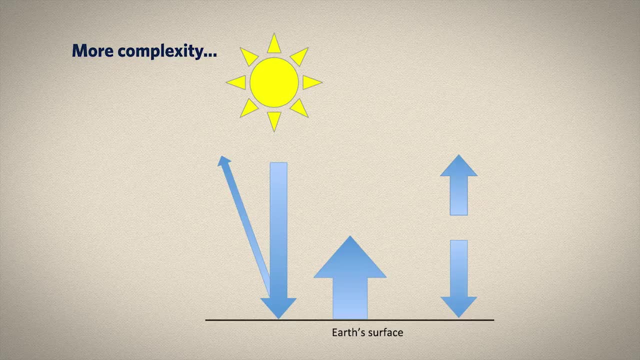 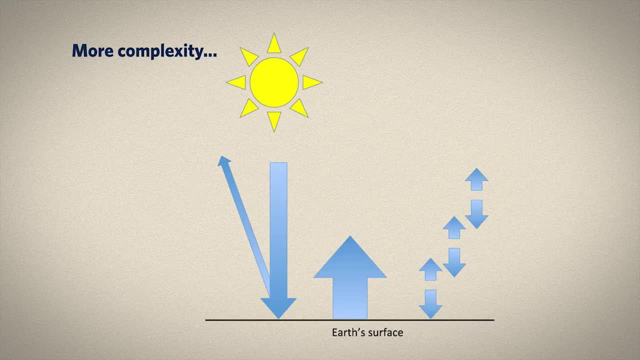 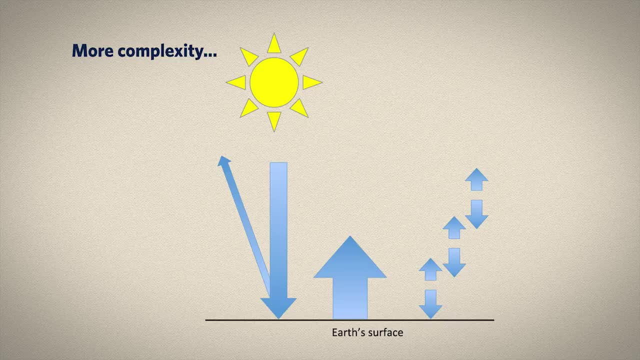 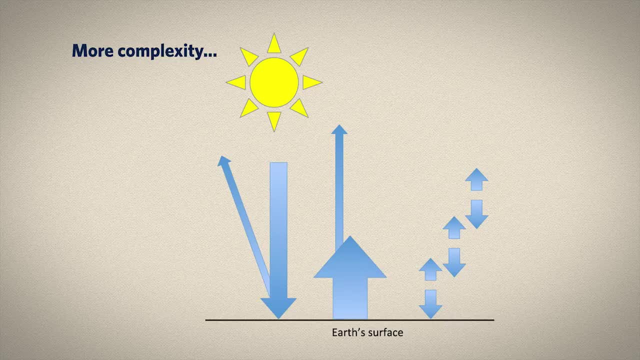 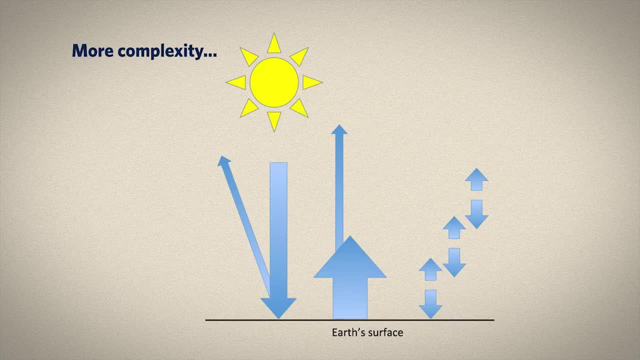 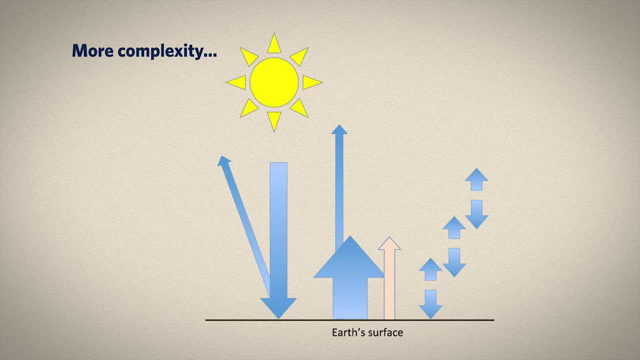 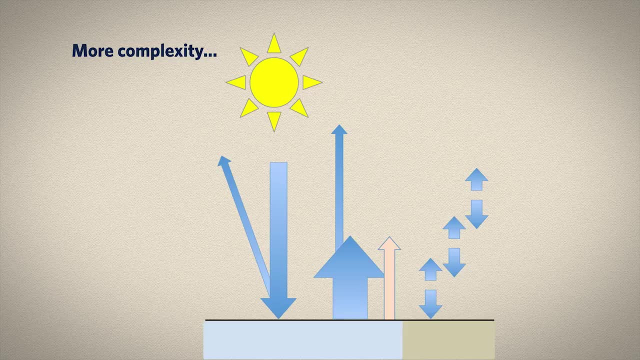 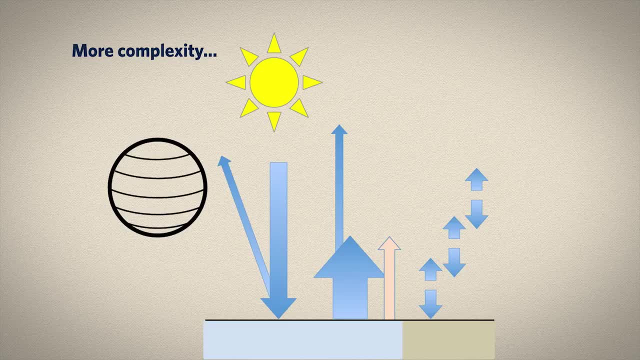 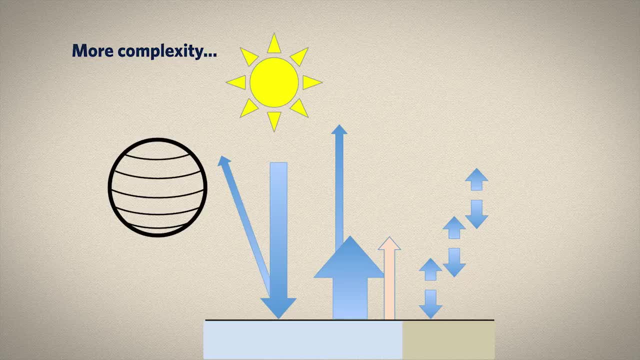 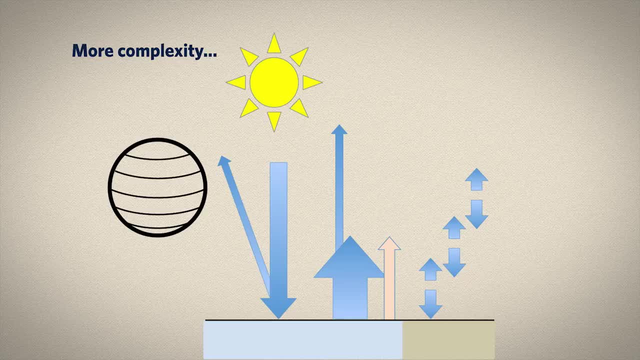 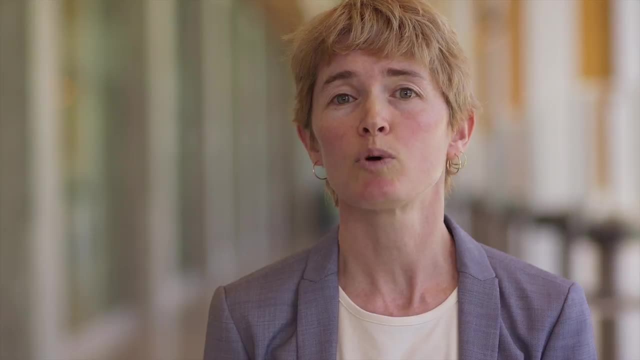 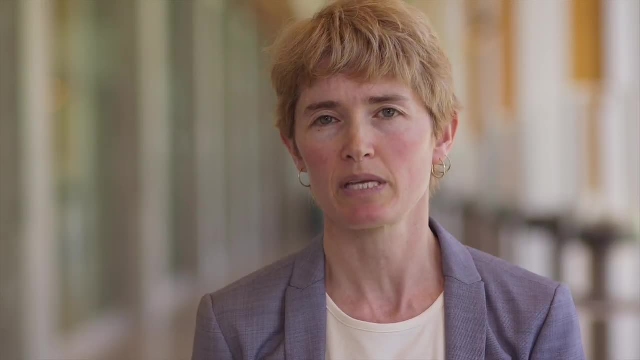 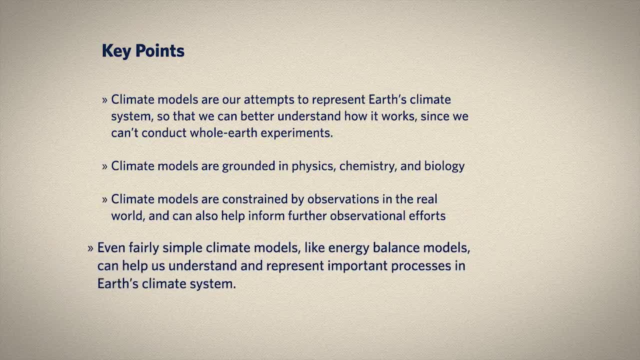 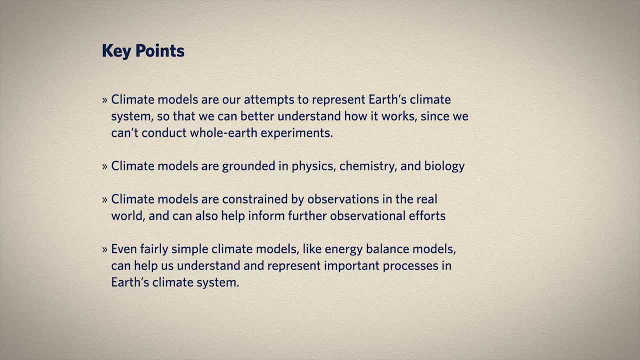 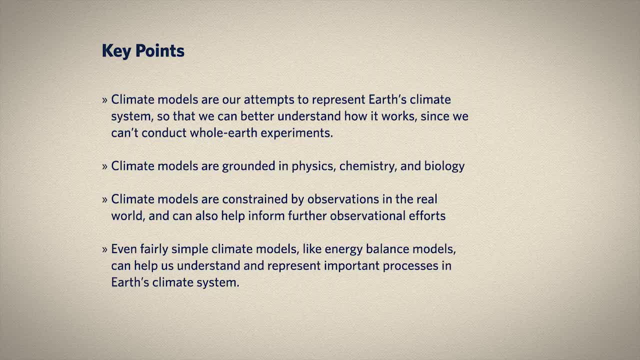 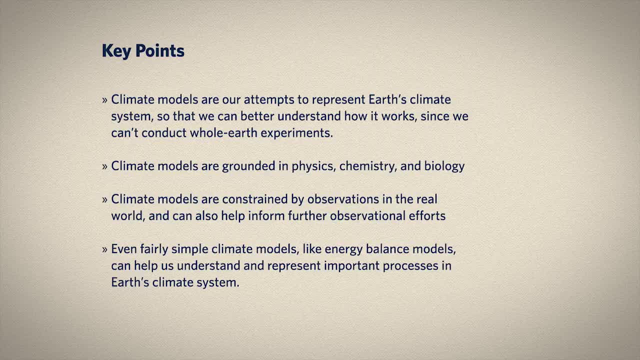 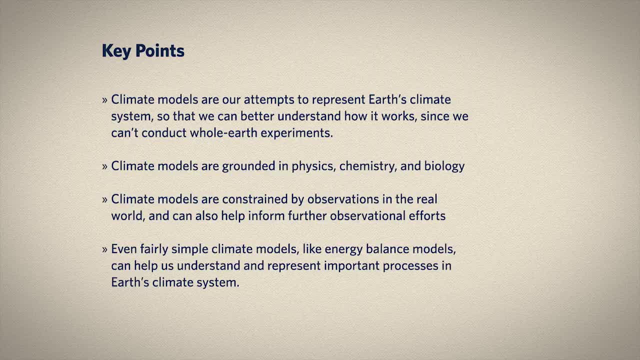 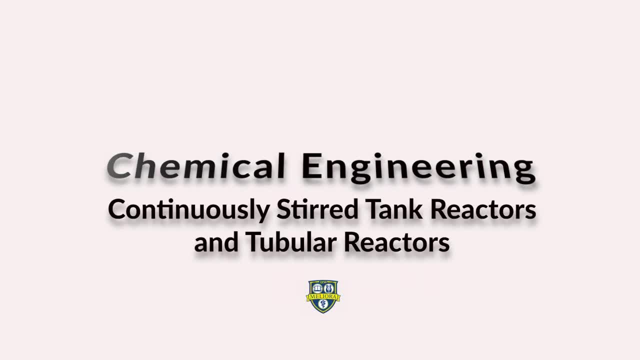 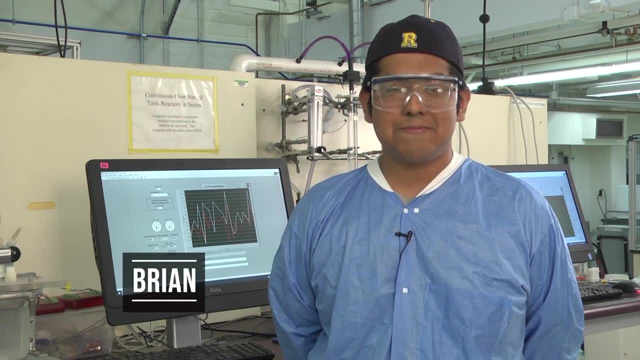 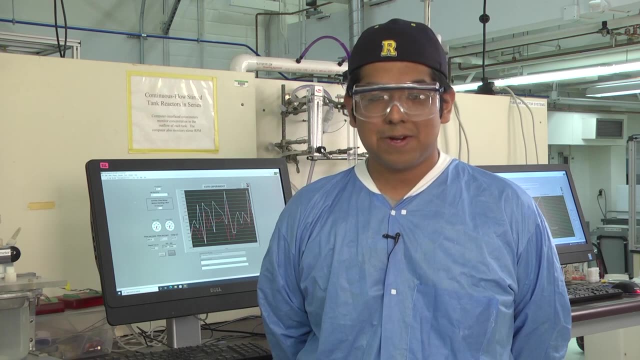 Hi, my name is Brian. I am a senior in the chemical engineering program at the University of Rochester, And today I'll be introducing one of the unit operation labs that you get to experiment on in your senior year laboratory course, And this one is the continuously stirred 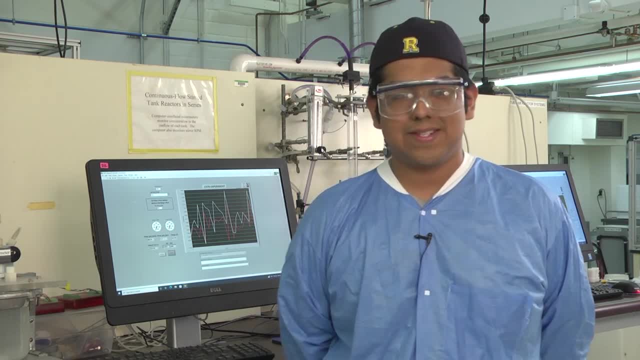 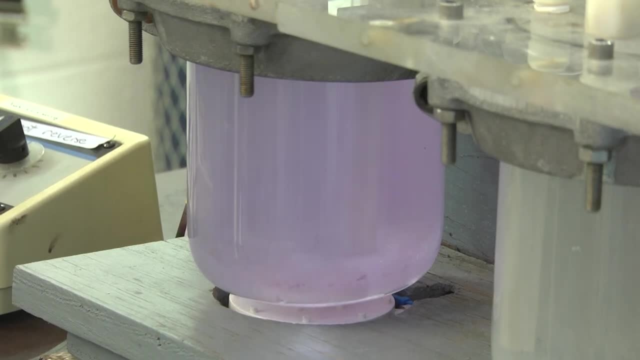 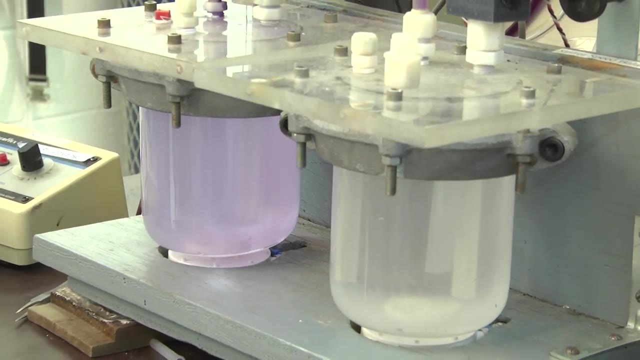 tank reactors, also known as CSTRs and tubular reactors. So what do we learn from CSTRs and tubular reactors? We learn how fluorides, component concentrations, reaction kinetics, mixing and deviations affect our real reactor system. 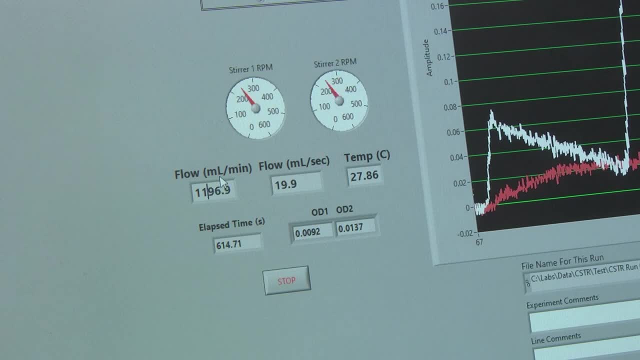 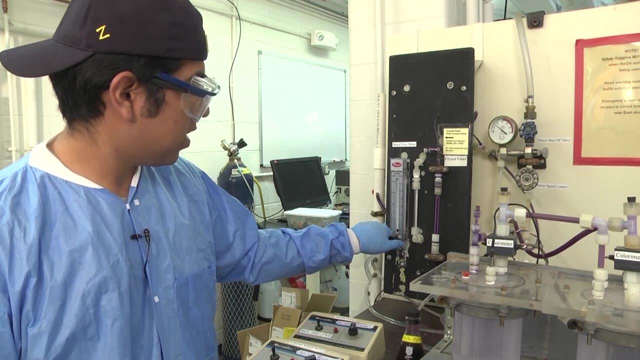 and also how much our real system deviates from an ideal system. This is done by modeling our reactions over time in two types of continuous reactors: CSTRs and tubular reactors. We do this to find conversion, residence time, distribution and reaction kinetics.